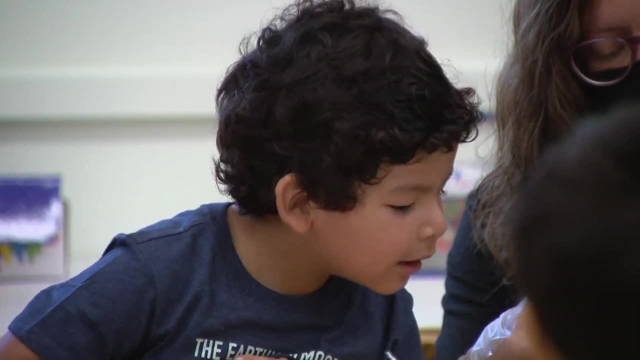 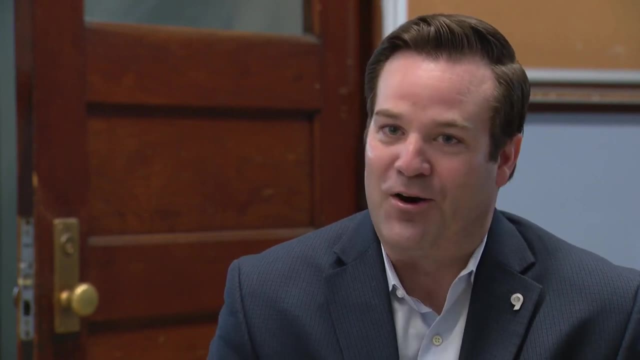 a chance for these three-year-olds to gain exposure and experience with education before the school year begins. Study after study has shown that kids who participate in pre-K are much more successful later on. Why is that? I want to say it's the cornerstone of the building blocks. 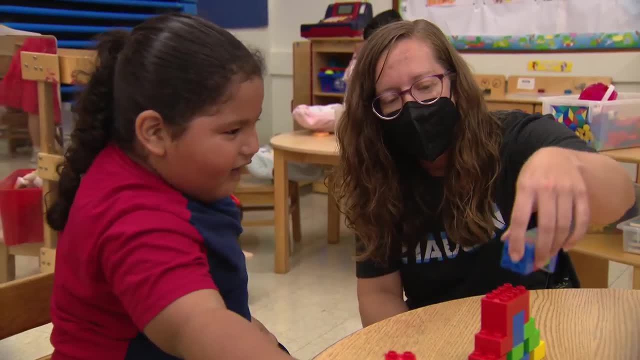 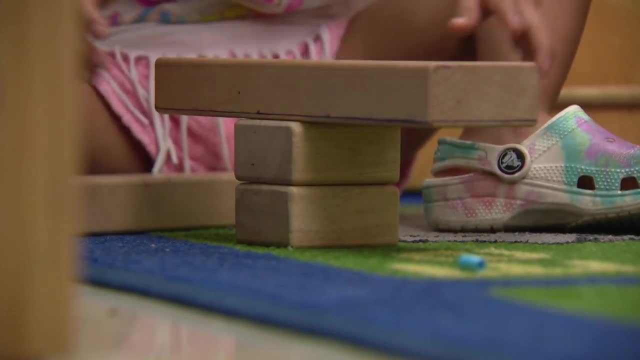 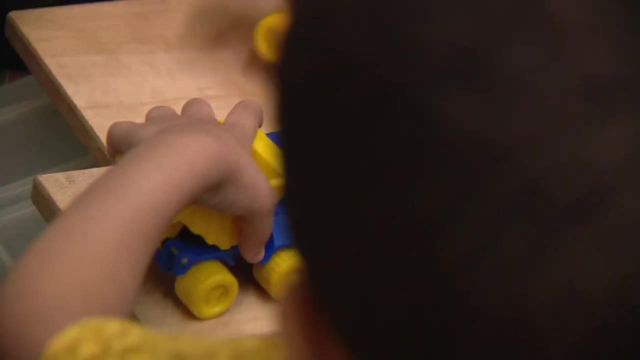 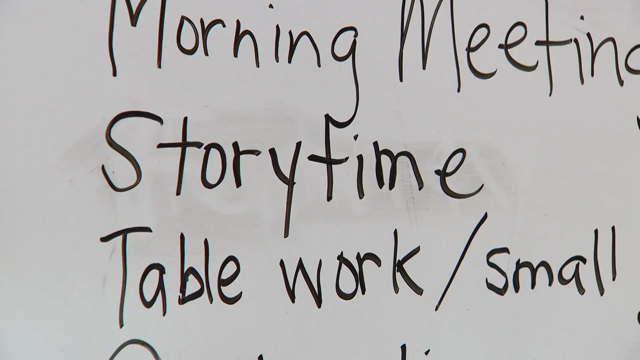 Basic but critical skills like learning routines, following rules and socializing with peers. Oh que paso? What happened? Oh, you want to turn too. The students are following a schedule from breakfast and clean-up to morning meetings, story time and table work. 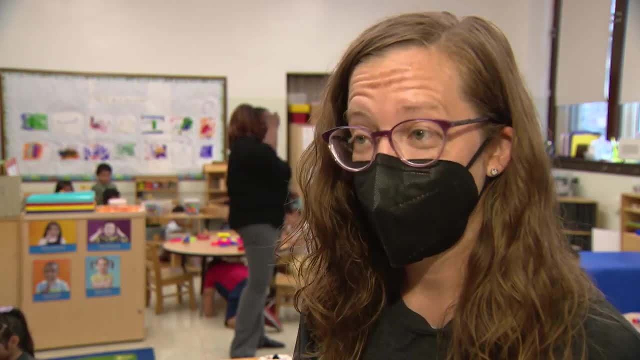 These things that seem very simple to us are very big skills, and they're not. as I said, A lot of these classes are done by kids who have had to spend the day in the classroom. The school starts August 22nd. It's right around the corner. 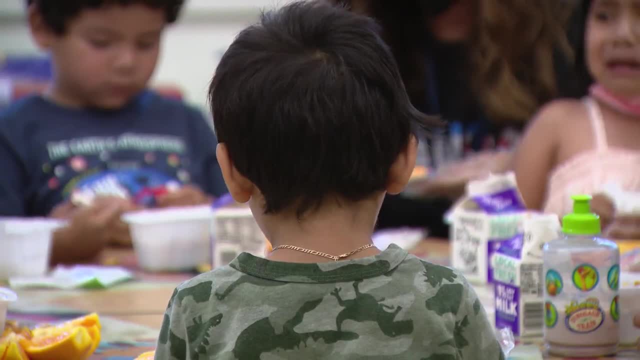 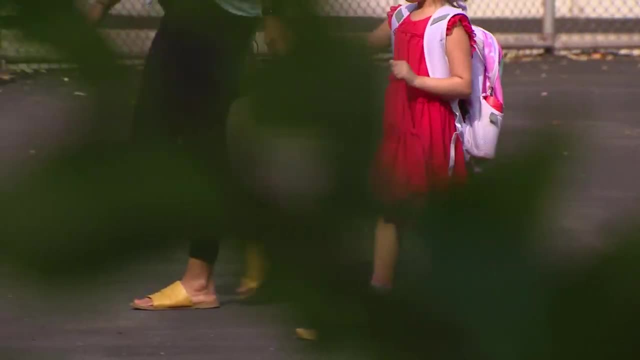 We still have seats available for pre-K- Early childhood education. chief officer Leslie McKinley says there are still 4,000 open seats for full-day preschool and about 1,000 open slots for the half-day program. It is open for everyone. 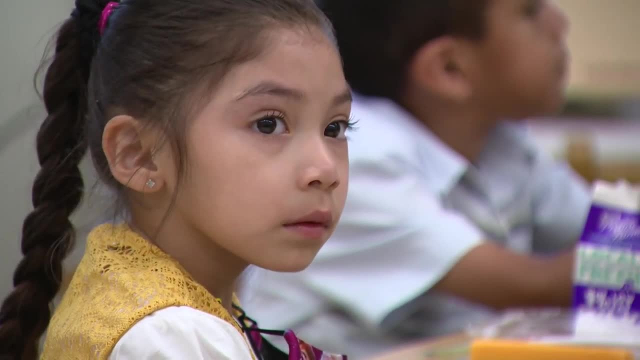 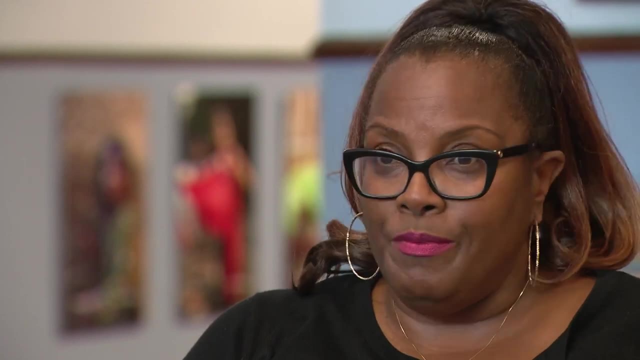 We are in over 350 elementary schools across the city. Families can apply to any school, So whether that's in the school district or outside the school district, Whether that school is close to home or close to work or close to grandma's house, you can. 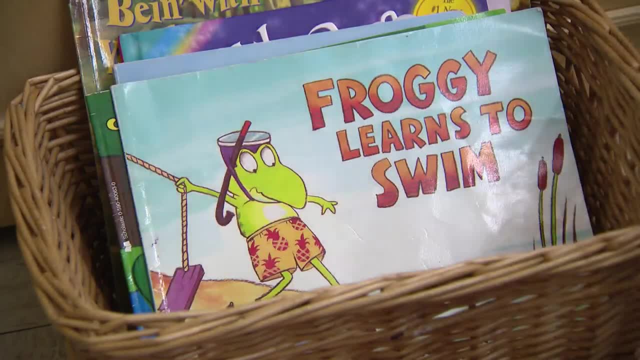 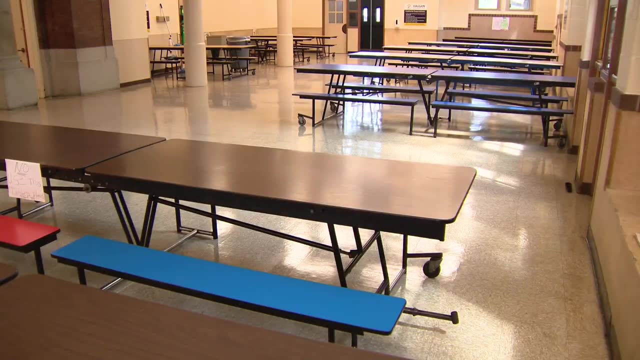 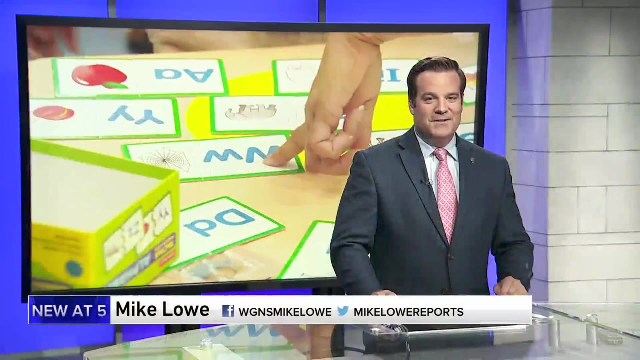 apply for that school. CPS says pre-K classes are one way to set your children on a path to success, even when the hallways are still on summer break. Sometimes it looks like an orchestrated chaos. that's what you saw today. So how do you enroll in a CPS preschool program? 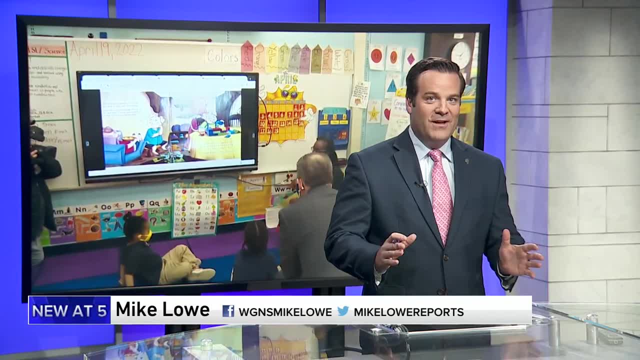 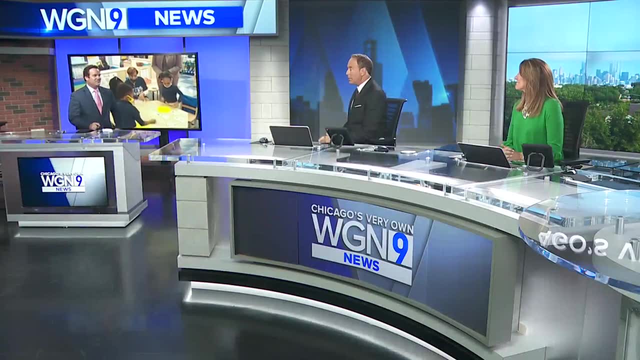 Well, if you have a three or four year old, enrollment is open all year round and we have a link with all of the information, the websites and phone numbers on our website at WGNTVcom. Do they usually have that many openings? is there some hesitancy? explanation for what's. 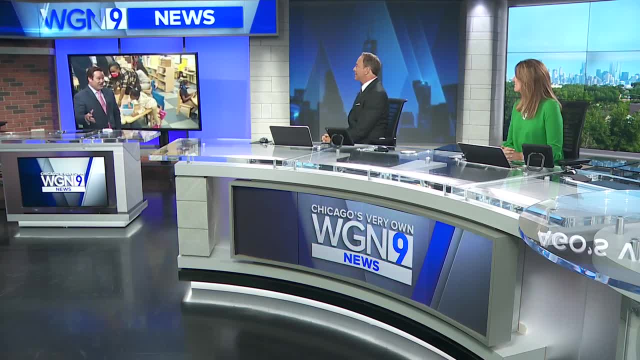 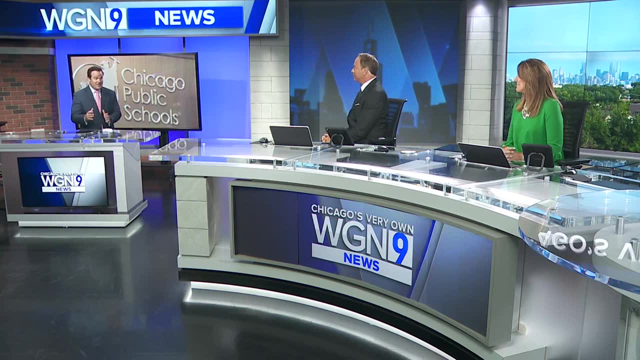 going on. There is some sense that people think you have to pay for this, but it is free and open to all. 4,000 full-time slots still available for next year and if you want to put your kid in a part-time program, 1,000 of those slots are still available.